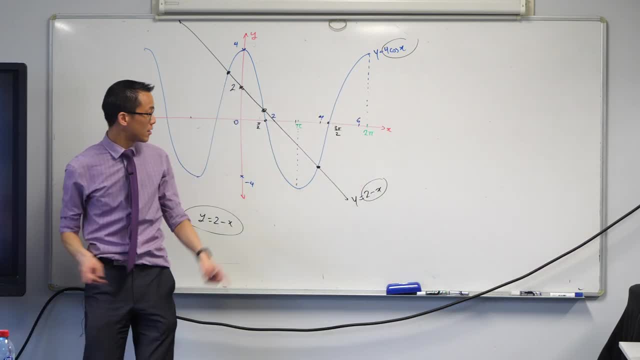 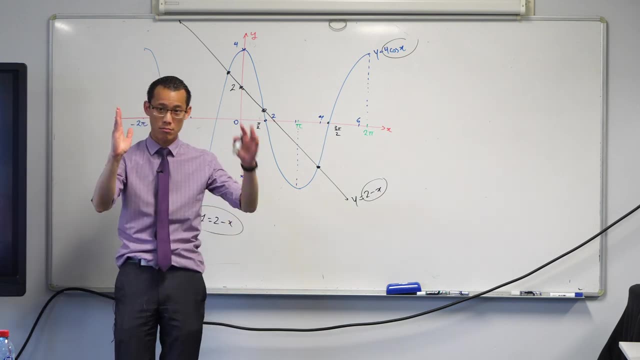 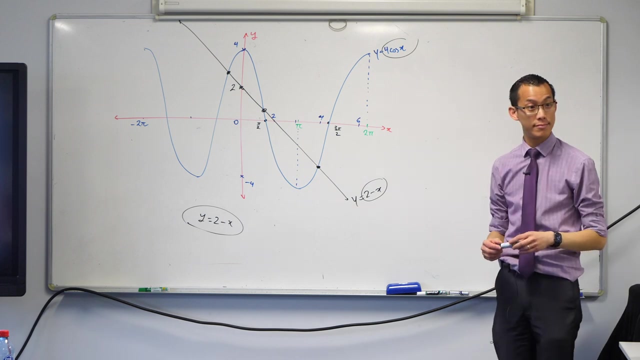 They've said, explain why those spots. even if you don't know exactly where they are, we can know they have to be between negative 2 and 6.. That's the goal, Perrin. So is it because after x equals 6 or x equals minus 2, the range of the 2 minus x is beyond 4?? 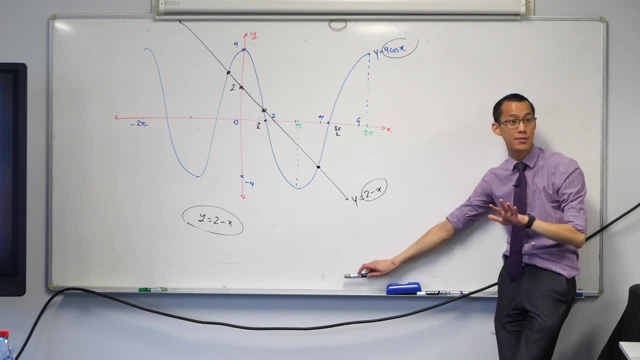 Ah, okay, Let's just pause for a minute- Pen's out of hands for a second- because I want to take Perrin's idea here and I want to make sure we're on the same page, Okay, Shhh, So Perrin, correct me if I'm misrepresenting. 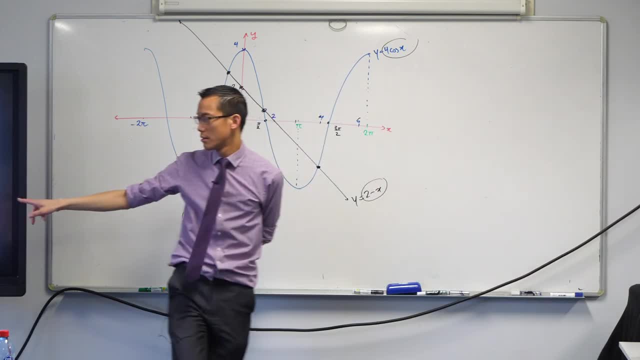 What Perrin just said was: after you go past x equals minus 2, you're going to have negative 2.. After you go past x equals negative 2 over that way, or x equals 6 that way. So here's like x equals 6, yeah. 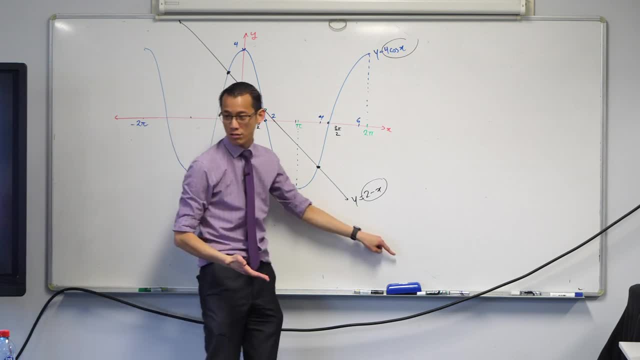 Look at what's happening to this graph. Do you see what's happening to it? It's just like dropping off the rock, right, And it's just it's plummeting, fine, It's going further and further away from this guy, right. 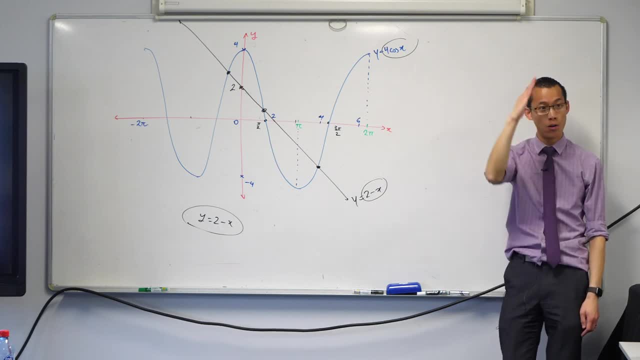 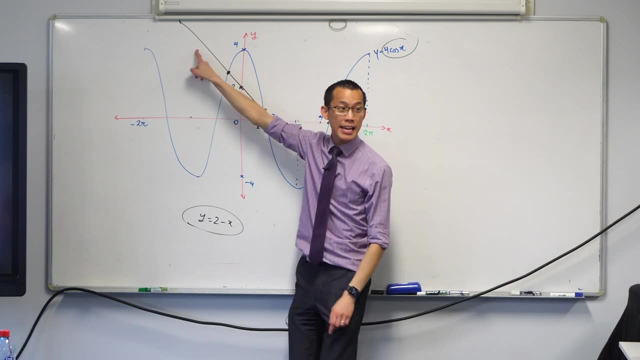 Do you see that This guy just happily stays between 4 and negative 4, just that's its home. But this guy's just like. I'm out of here, right, And the same thing happens over here, right. Negative 2: off to the left. 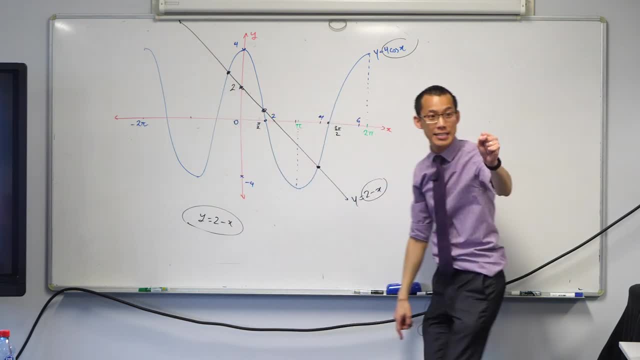 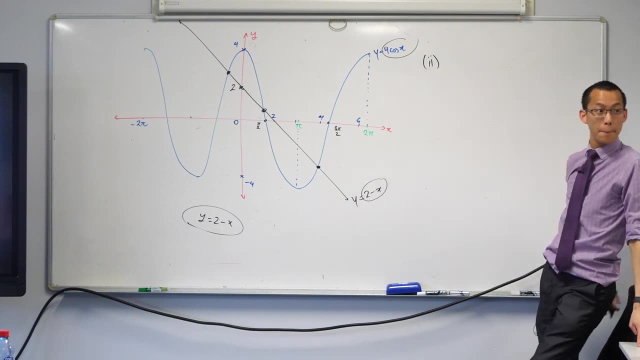 It just goes in the opposite direction. So this idea is exactly right. I'm going to show you how to express that. Okay, so let's do part 2 together, Sir. Yeah, Sir, wouldn't y equals 2 minus x also end at 2 pi over negative 2 pi? 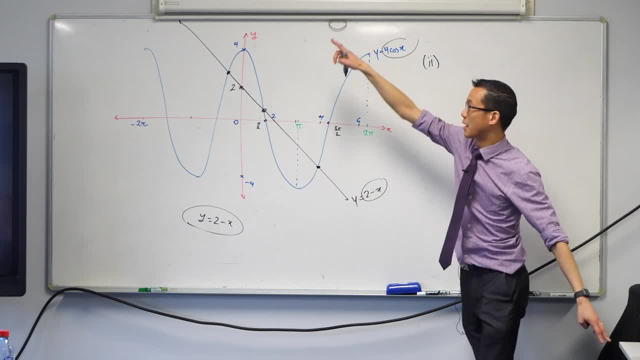 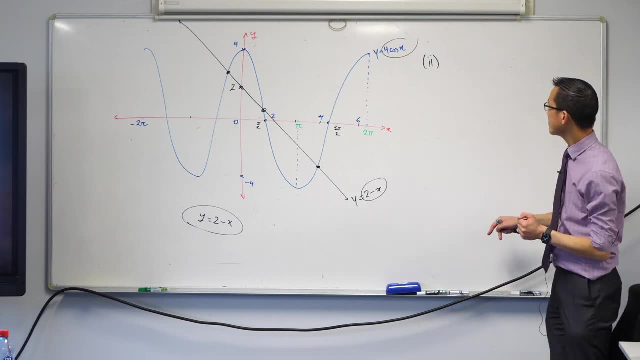 Yeah, so in fact, this graph would go up to here, but I've gone off the board, so sorry, Okay, Alright, stay with me. So here's how we're going to prove it. We're going to consider, and this is literally what I would write: 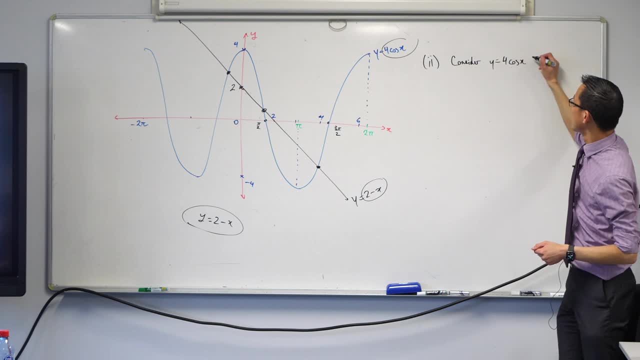 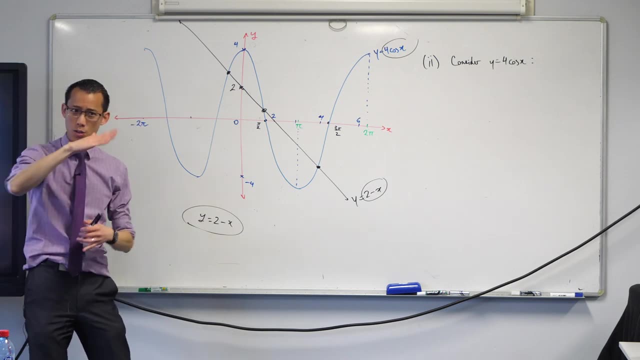 Okay, We're going to consider this trigonometric graph. Okay, Remember, the whole issue was it sort of stays within this range and it never goes outside, that, It never strays. Okay, So what is sorry? can you wait? 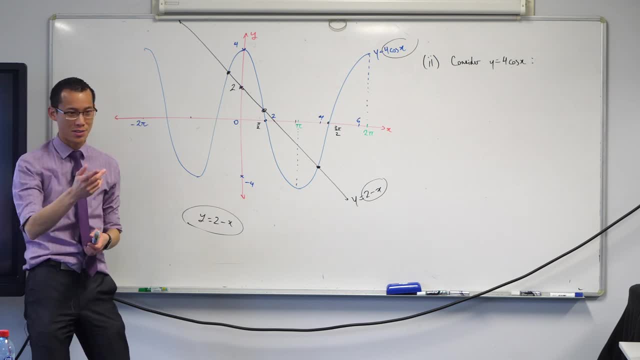 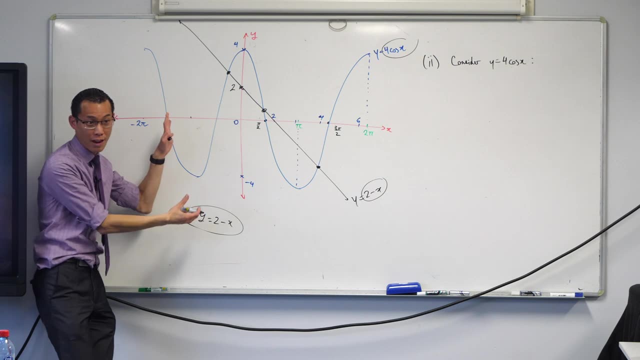 No, can you wait? Thank you, Just sit down, You'll have time. I want you to articulate for me- It's on the graph, It's probably on your graph- What is the actual range of this 4 cos x function? 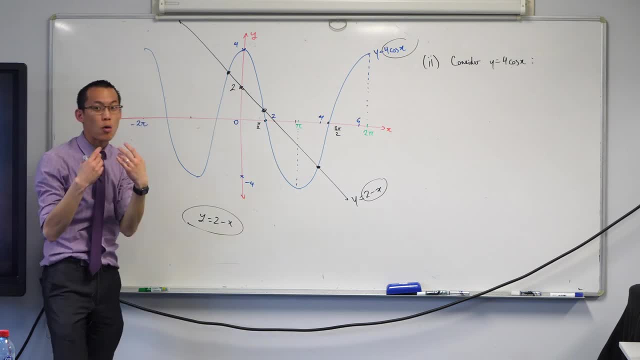 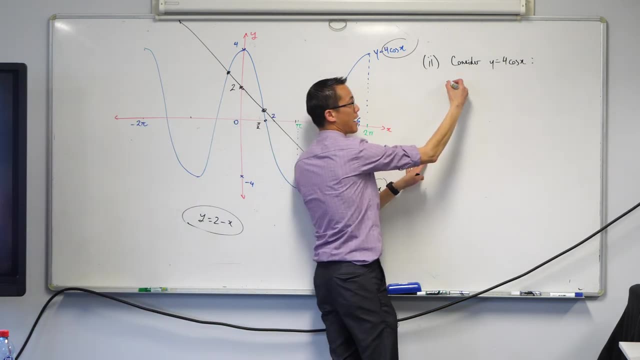 8.. 8? Have a think. Range means where do you start and where do you end. It's negative 4 all the way up to 4, right. So how we write that? we would say negative 4 and 4, they're like your boundaries, right. 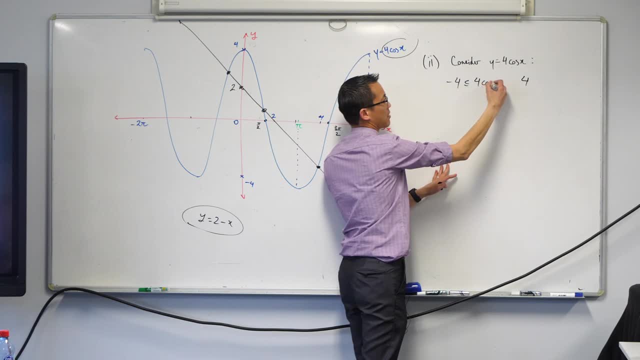 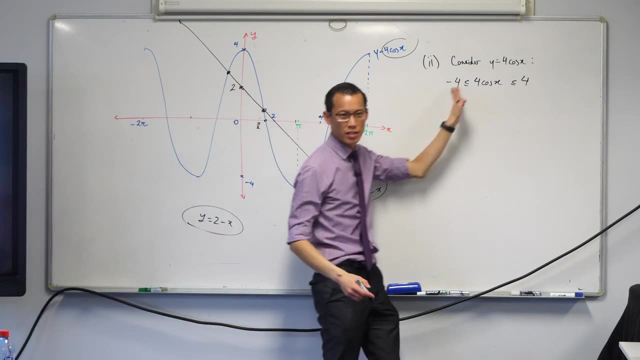 So I'm going to use an inequality notation. I'm going to do it like this: Are you okay with that? Yep, So I always think: well, I always go from smaller to bigger. You can see that in the direction of the inequalities, right? 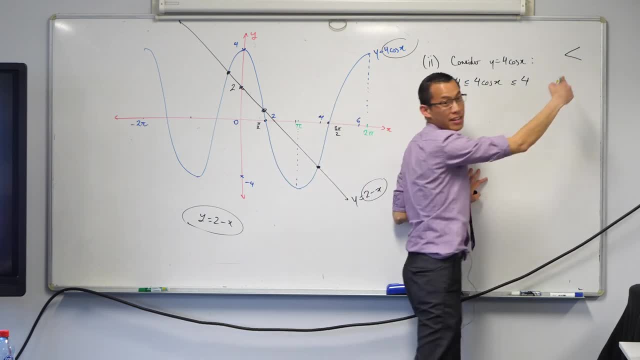 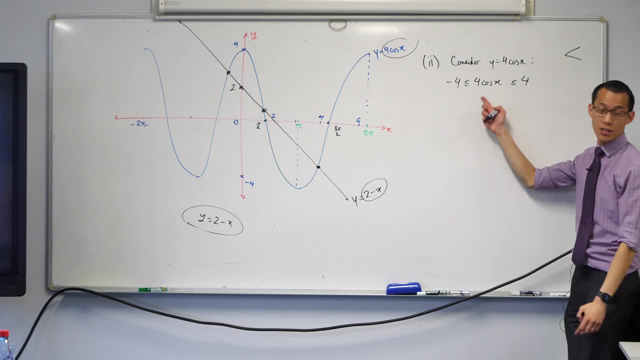 The inequality itself. it's got the small end on one end and the large end on the other. Okay, You with me, So we can say this is true from the graph, even from the definition of cosine. Thumbs up, Okay. 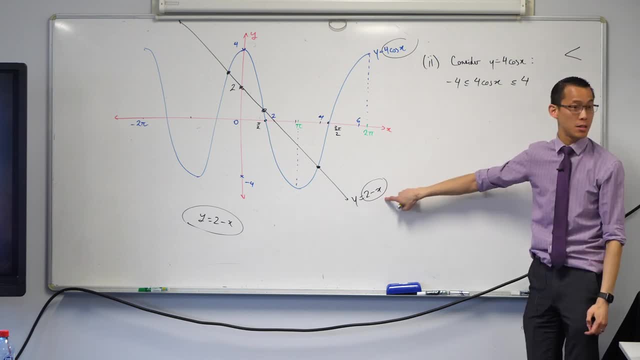 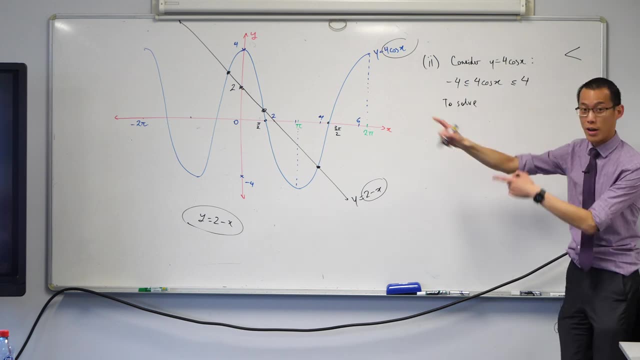 But what they're asking for is this straight line to be equal to that trigonometric graph, Right? So, therefore, to solve that equation that they gave us, Okay, That equation that they're giving us, Right, The one in the question. 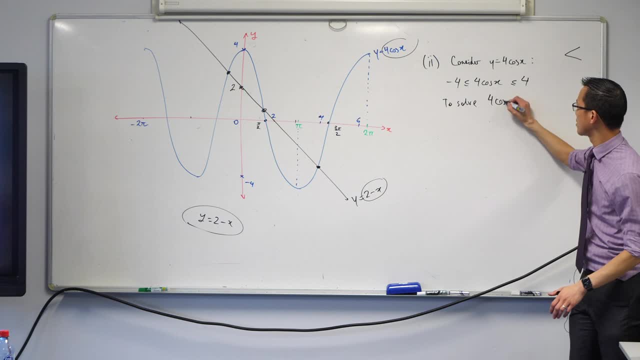 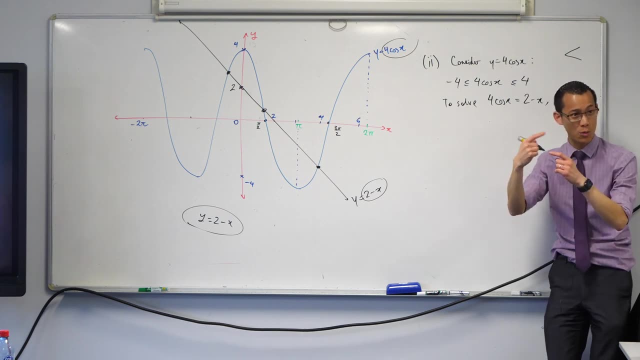 Is it 4 cos x first? It is, isn't it? Yep, To solve 4 cos x equals 2 minus x. Okay, There's a really big leap in thought here, so watch closely. If you want this thing to equal that, then this has to live in that same space. 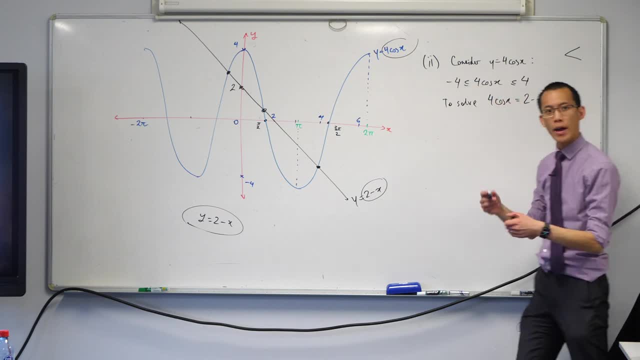 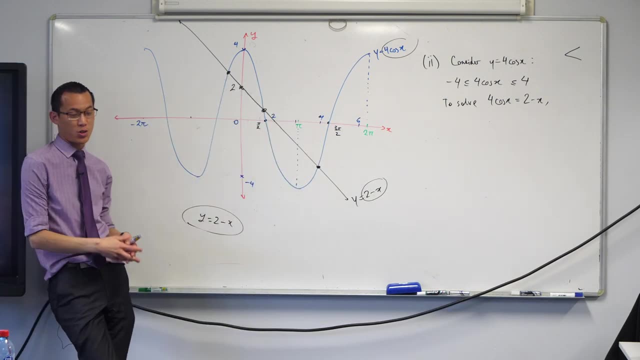 Do you agree? Right? It's like, oh, when it did it click for you? Okay, So when are you going to see Mr Wu at the shops? Well, he only ever goes to the shops at Castle Towers, or whichever they happen to be. 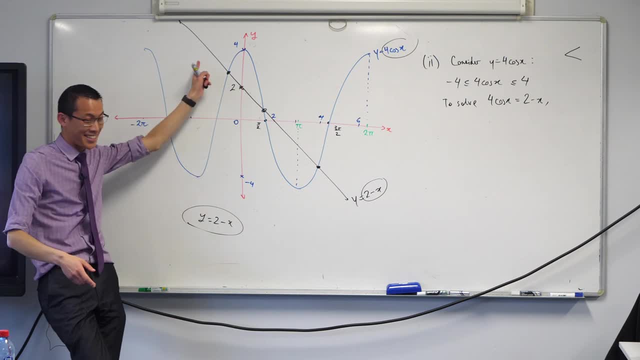 Right, If you want to find me, if you want to bump into me at some point, intersect with me there. you're going to have to go to those shops. Does that make sense? Because I'm lazy, I don't want to drive far away. 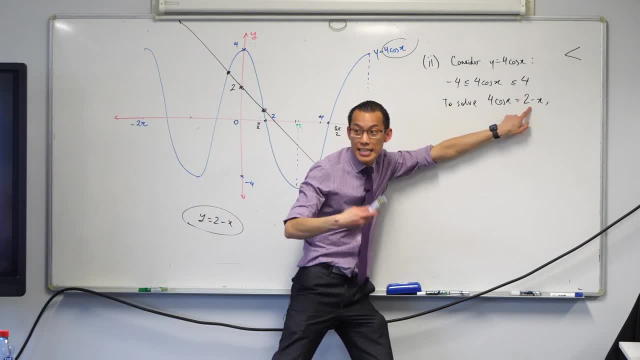 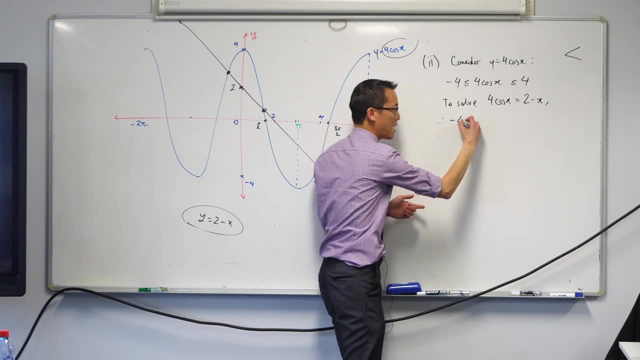 Okay. So I need this thing to live in the same space as this one. You with me. So I'm going to say, therefore, it's got to be between negative 4 and 4. Okay And 4. Right. 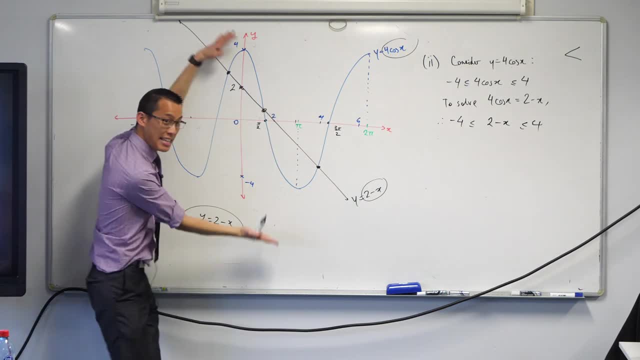 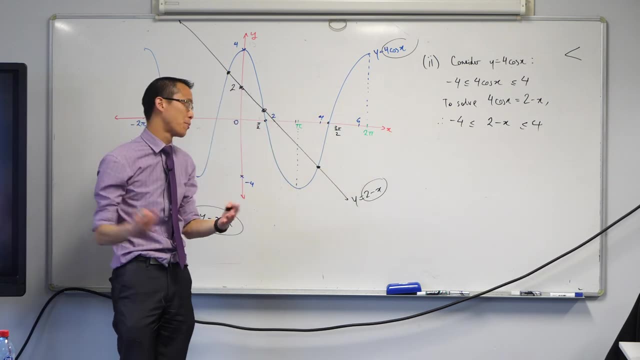 That's what this 2 minus x has to do. It has to live in this restricted range. Does that make sense? Now, that's a. that's not much to write, but it's a big mental step. You pretty much actually have done this now, because where are we trying to get to? 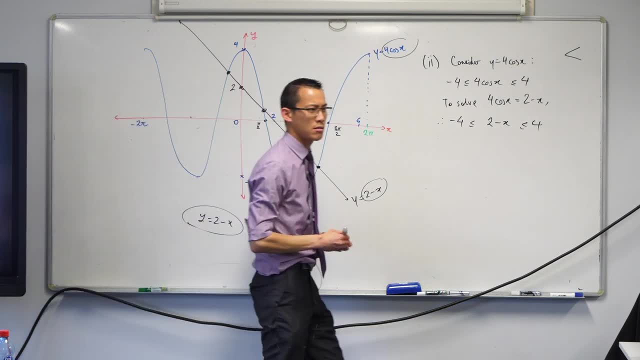 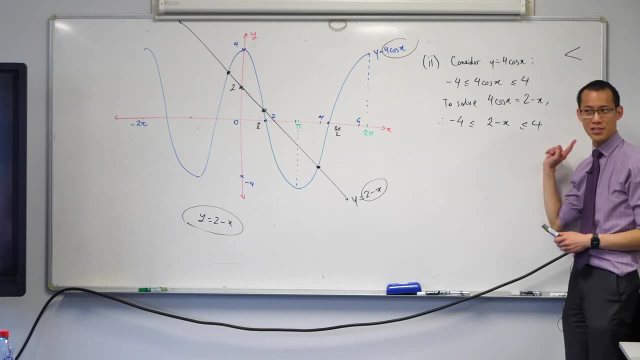 We're trying to get to negative 2 and 6.. Where do you think they come from? negative 2 and 6? What can we do with this thing? Any suggestions? I want to solve for x right Now. it's weird to solve this thing for x because x is in the middle. 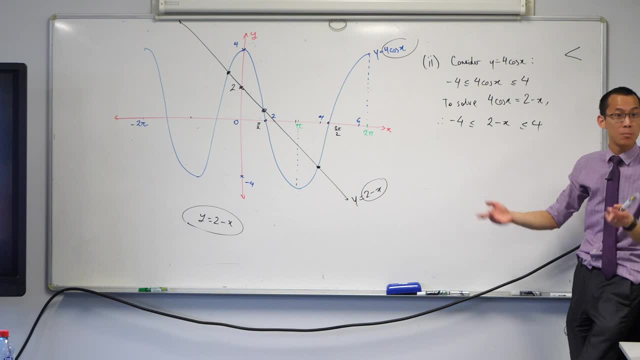 Ugh. Another reason why this is such a hard question, But we can still do it. We can still do it. 2 minus x: I want to get the x by itself. Any suggestions? What am I going to do first? 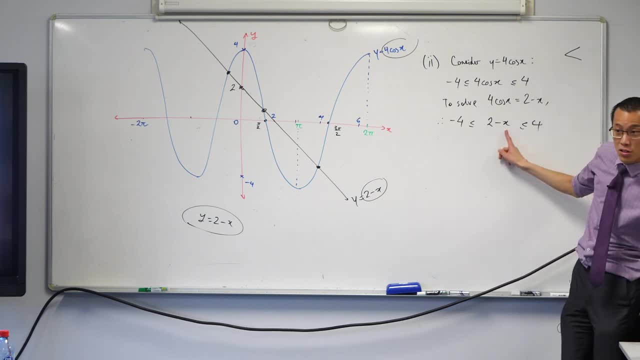 I'll subtract 2.. Now, subtracting 2 from this means I don't just subtract 2 from that, I have to subtract 2 from everything, Right? So I'm going to subtract 2 from all. did you see it? 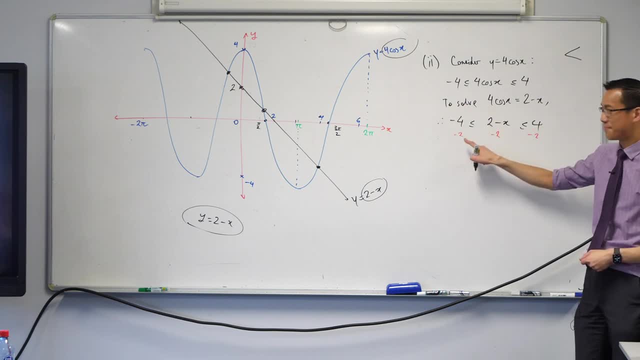 Okay, good, Right. So over here on this side I get negative 6.. What do I get in the middle? Negative x, Negative x. thank you, What do I get on the right hand side? 2. 2. 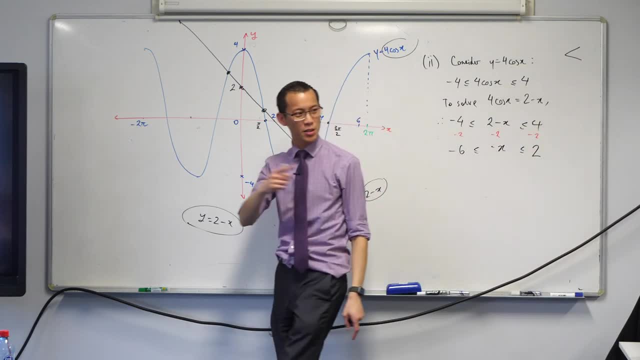 You're like: ooh, wait a second, I wasn't supposed to get negative 6,. I was supposed to get positive 6.. But that's okay, because I've got to deal with this minus sign as well. So what do I do now? 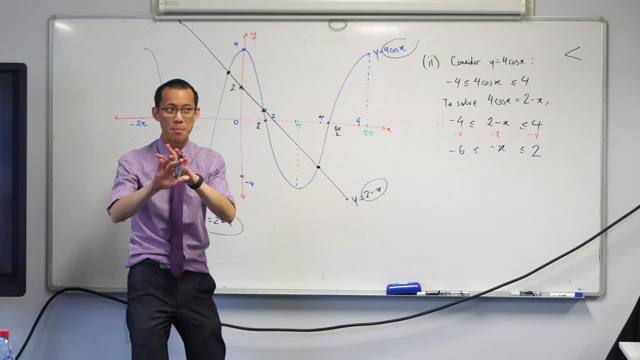 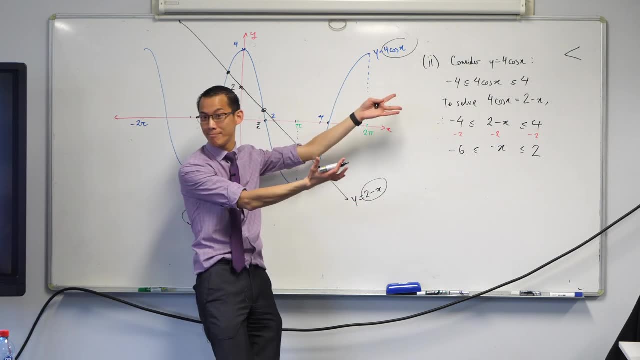 Divide by minus 1.. Think carefully. I had a bunch of different answers there. Max, what are you thinking? Divide by minus 1.. If I divide by minus 1, or, equivalently, multiply by minus 1, that'll do. 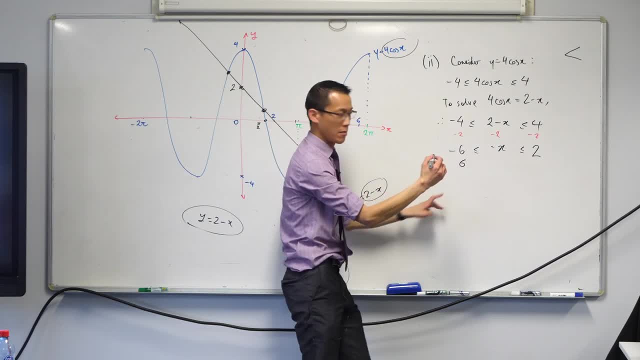 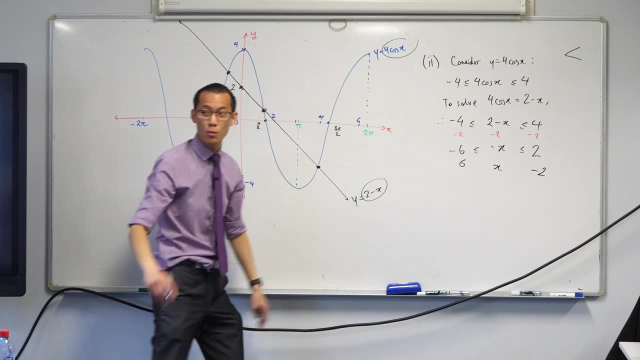 Okay, So this will become 6.. This will become x, This will become negative 2.. That's good, But there's one thing you have to be super careful for. Remember we told you guys, inequalities are like equations in many ways. 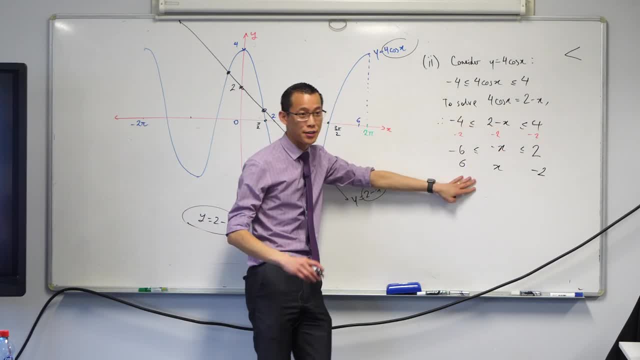 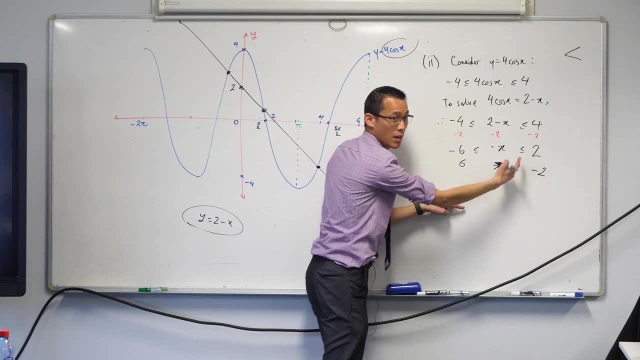 You can do the same thing to everything, it's all fine, But they're different in some very important ways, like right now: Yeah, my inequalities are going to go different directions. So these are less than or equal to's. They're going to become greater than or equal to's.